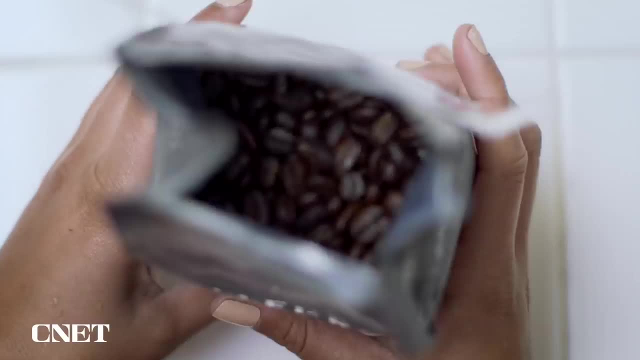 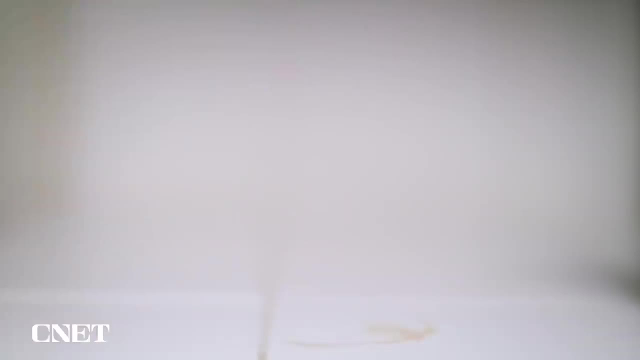 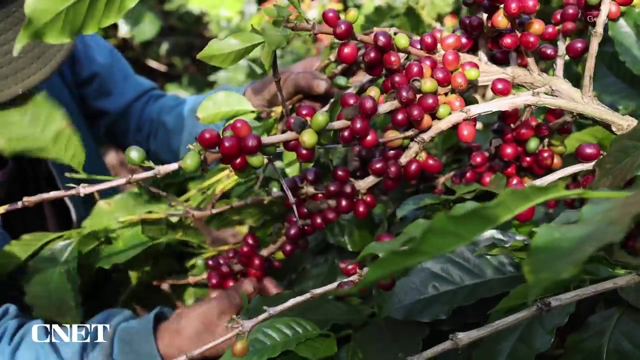 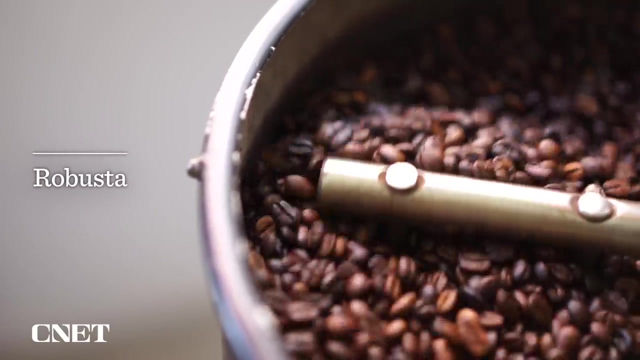 Your morning cup of coffee is in danger. Not your specific cup of coffee, but the beans that make it. The multi-billion dollar coffee industry relies on just two species of coffee plants. Robusta is known for its complex flavor profile, while Arabica the more popular coffee varietal. 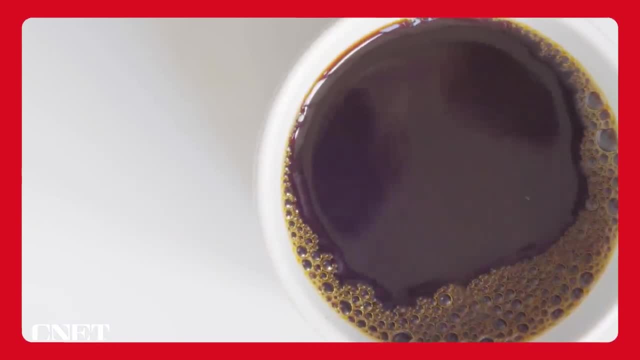 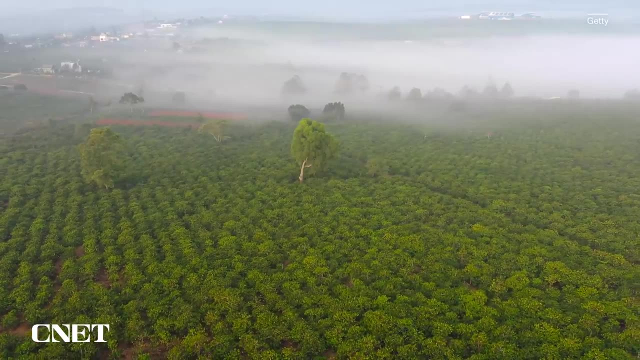 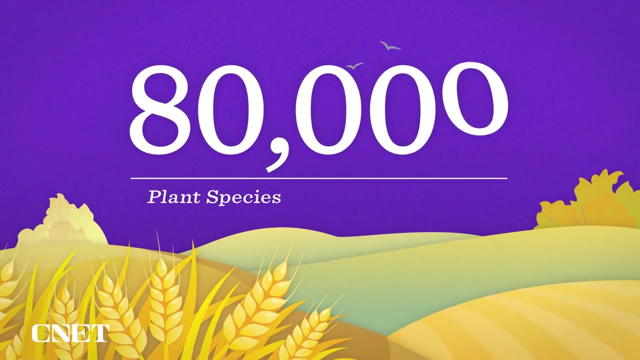 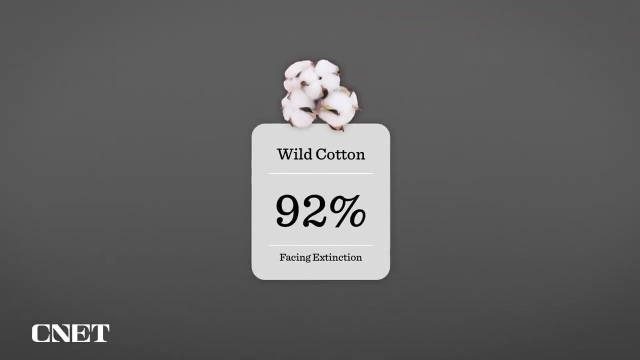 is on the endangered plant species list. Coffee plants are one of dozens of important crops threatened with extinction. Experts estimate roughly 80,000 plant species. one in five are at risk of extinction. Wild cotton is the second most threatened, with 92% of species at risk of disappearing. Three in five. 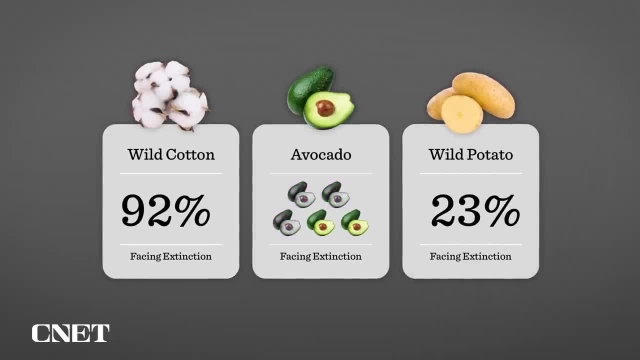 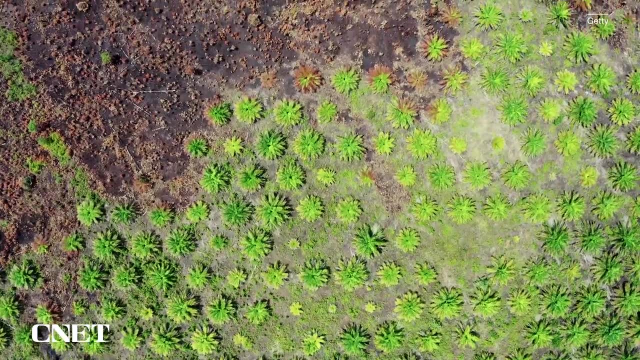 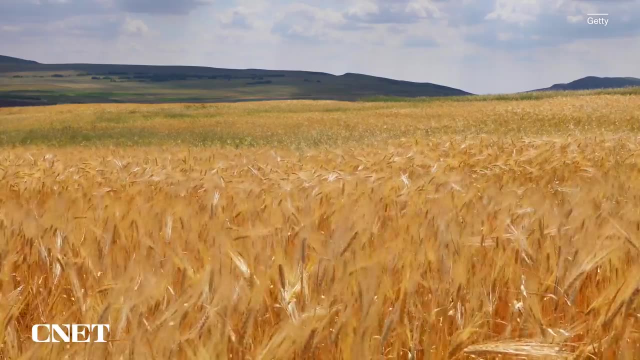 avocado species are at risk and 23% of wild potato species are facing extinction. Climate change and deforestation threaten the wild varieties of these popular commercial crops, which doesn't directly affect the produce availability in your local grocery store. But if the wild varieties of these plants are in danger, their commercially grown relatives. 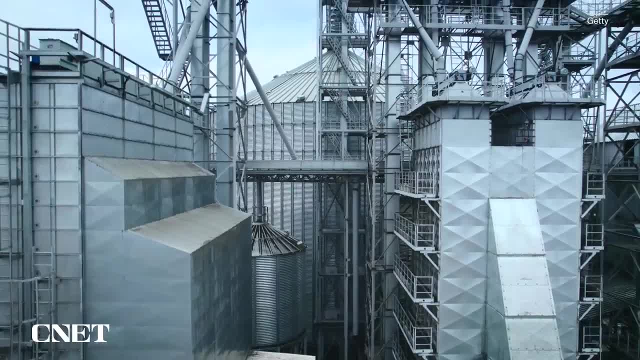 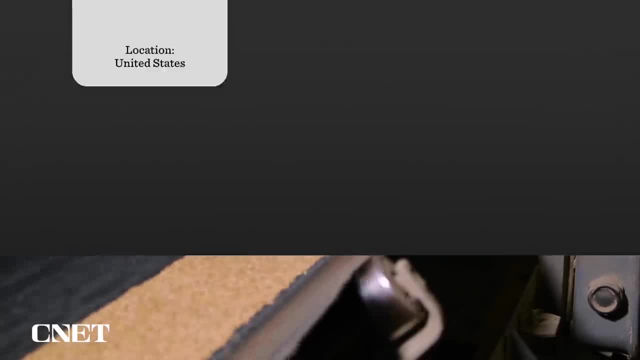 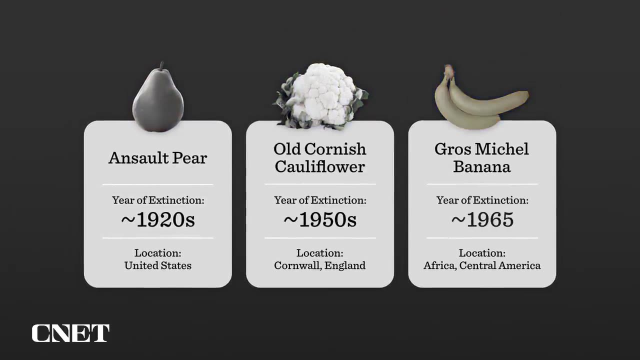 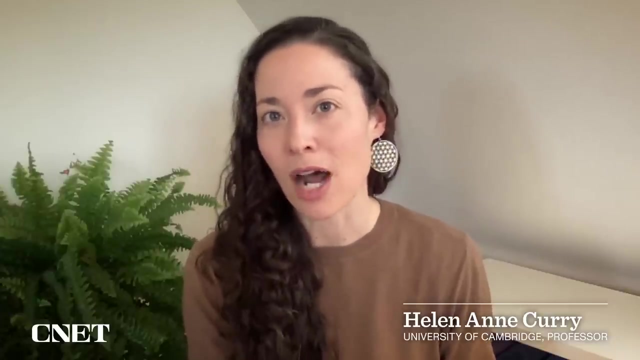 are too. This is because farming practices have become increasingly more industrial. As a result, humans have lost significant crop diversity. Crop diversity, The full spectrum of farm plants and the related wild varieties, no longer exist in industrial agriculture. This is a worry, because we tend to think that growing different kinds of off crops growing 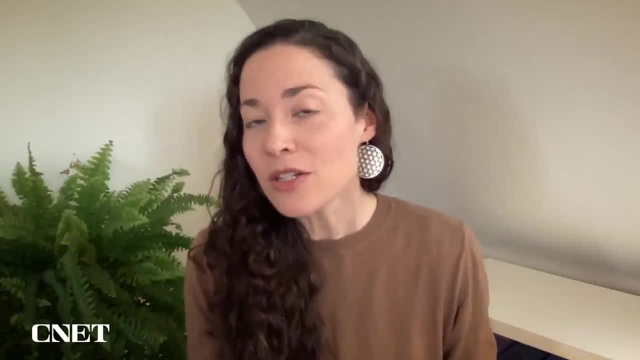 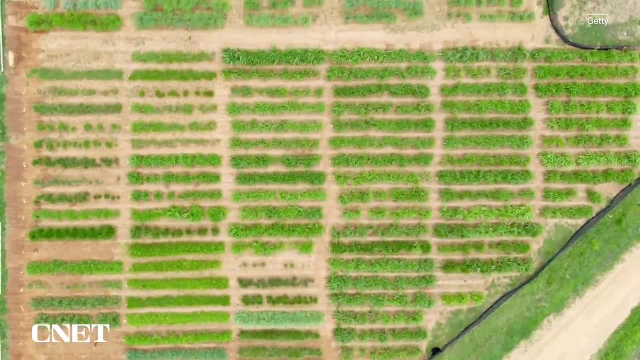 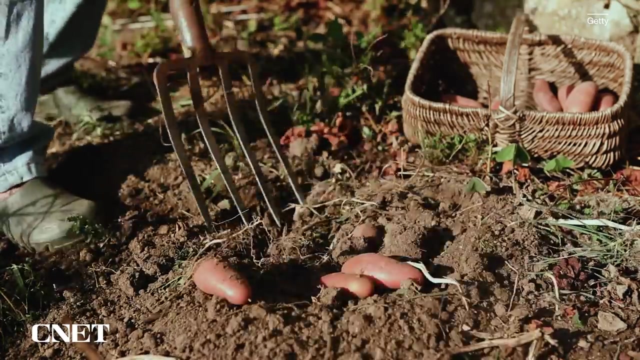 crops that are different genetically, as well as a wider range of species of crops, is a nice insurance policy if something goes wrong, say, or unexpected, with кοιмığı, climate changing or with unusual weather patterns in a particular year, or with new kinds of diseases or pests. the 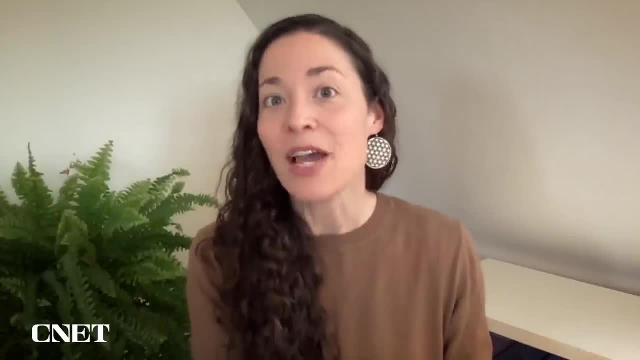 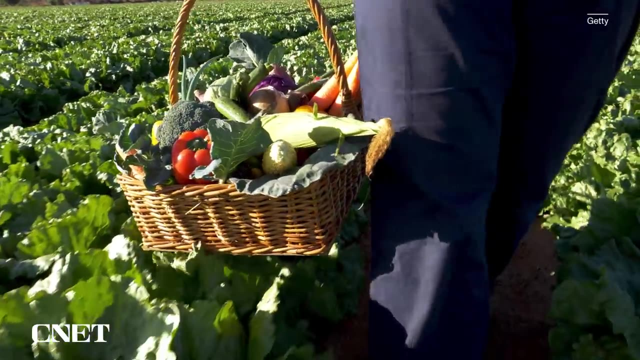 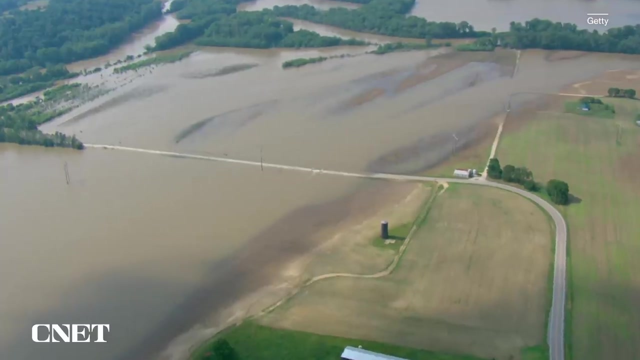 more heterogeneity right. the more differences we see within farm fields and across farm fields, the more opportunities we might have for resilient crops to survive and thrive, even where our vulnerable ones fail. Climate change impacts and risks to global crops and the production system are becoming increasingly complex and more. 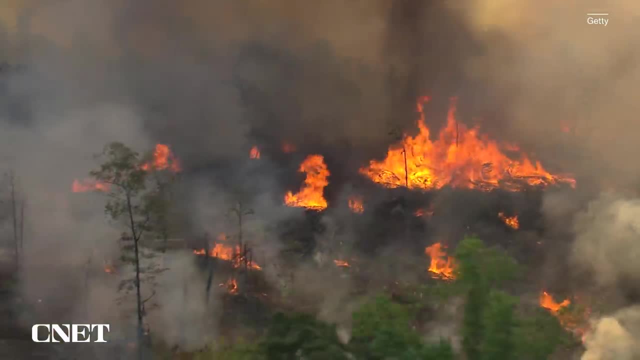 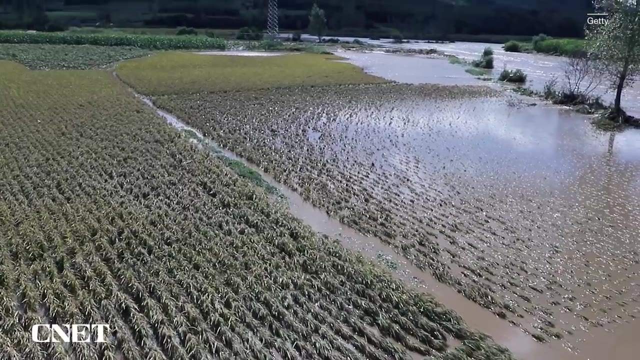 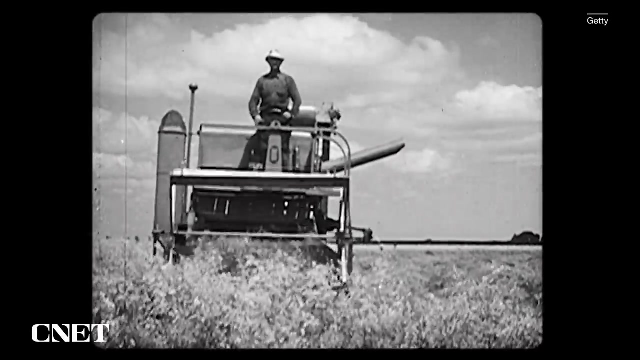 difficult to manage. According to the 2022 IPCC report on climate change, rising temperatures increase the risk that the agricultural industry will suffer simultaneous crop losses in major food producing regions. The loss of crop diversity started in the early 20th century, during what's. 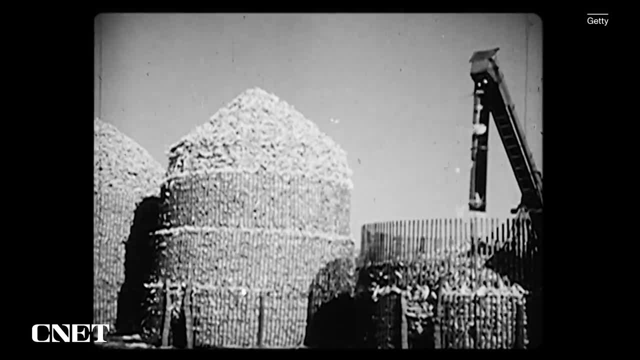 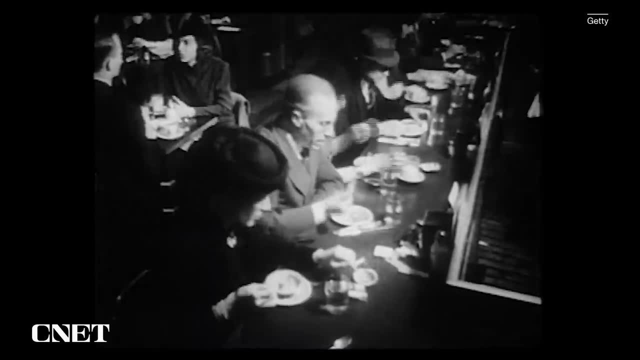 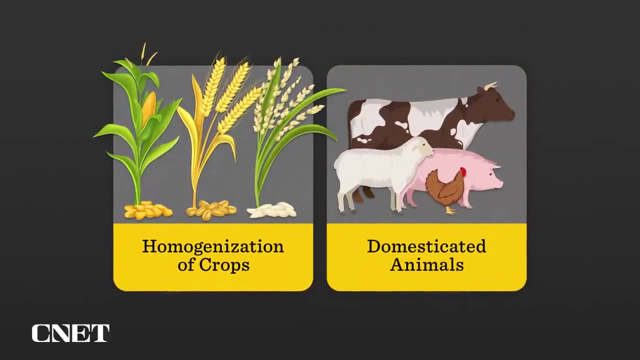 known as the Green Revolution, when farming practices shifted to high yield crops like rice, wheat and corn to help farmers survive. Farmers feed a surging global population at lower cost. However, a century of selective farming practices has led to a dangerous lack of biodiversity in our foods. 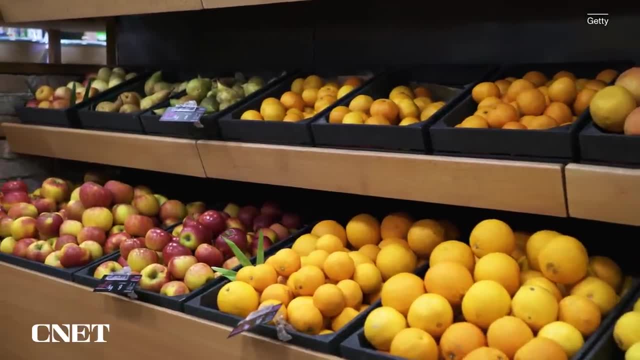 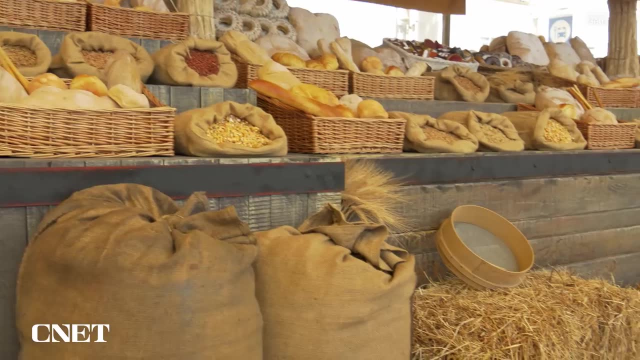 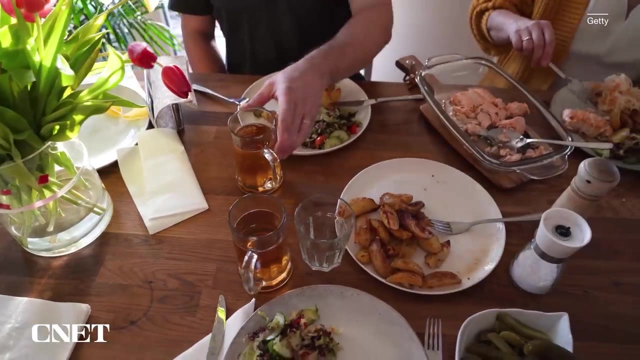 The diversity of crops that we've come to rely on, aggregated globally, have tended to diminish. We rely a lot on a handful of key commodity crops, So things like corn, wheat, rice potatoes- the things that immediately come to mind As items you would see on your dinner plate- are likely to be on. 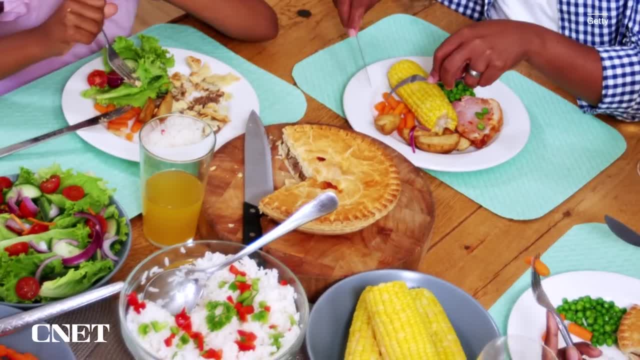 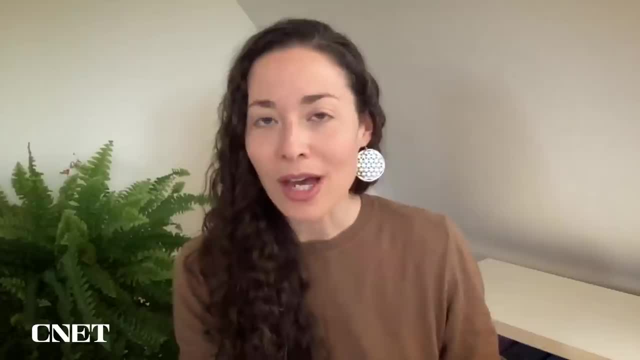 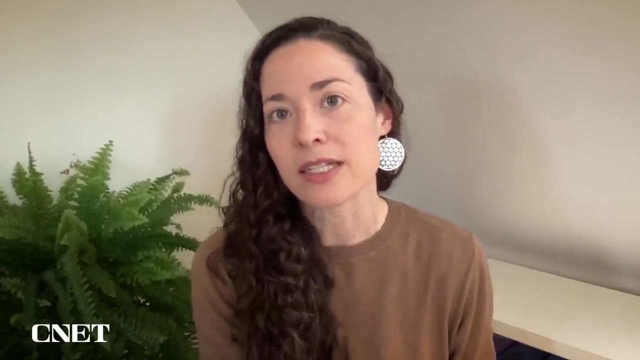 the list of species that other people around the world tend to consume and eat. But there's another kind of crop diversity that people worry about, which is a diversity that occurs below that level. So people might refer at times to the genetic diversity of the crops that we eat. 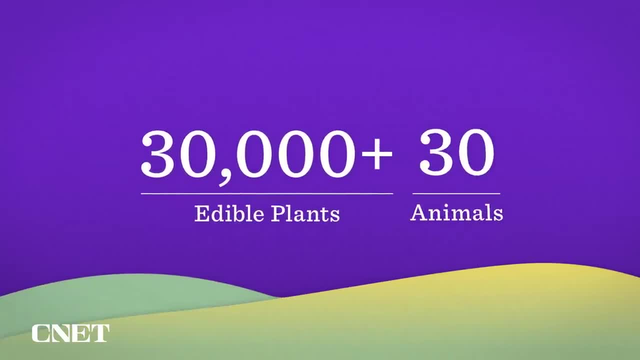 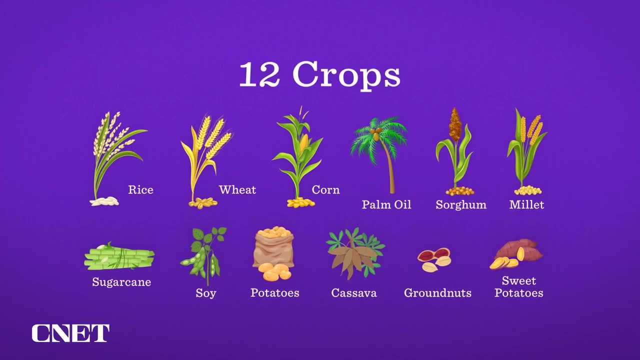 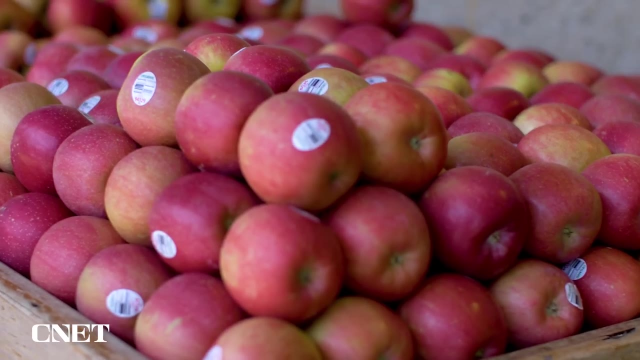 Historically, over 30,000 edible plants and 30 animals have been domesticated for food around the world. Today, over 75% of the global food supply comes from only 12 types of plants and just five animals. Relying on only a few crops for food poses challenges to our 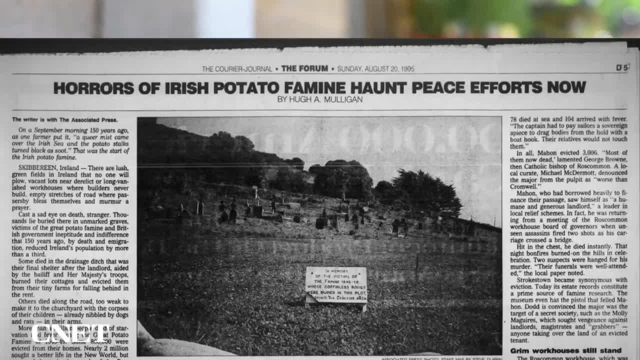 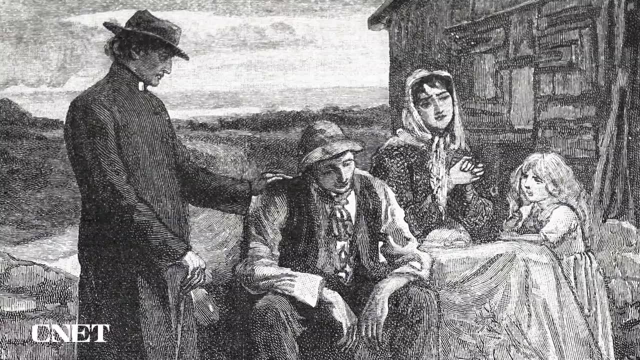 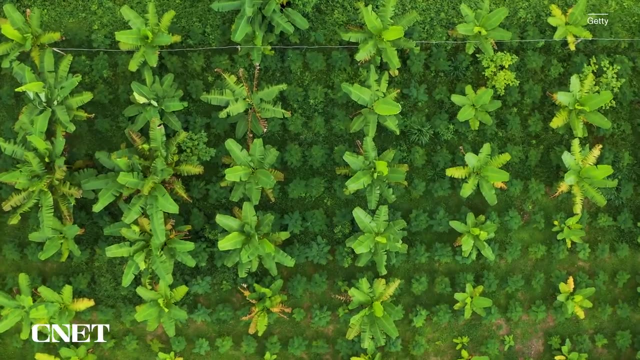 health, our food supply and the farmers who grow them. History shows us the dangers of relying on single varieties of crops. The potato famine in Ireland killed a quarter of the country's population when a potato blight wiped out potato crops all over the country. More recently, Panama disease is. 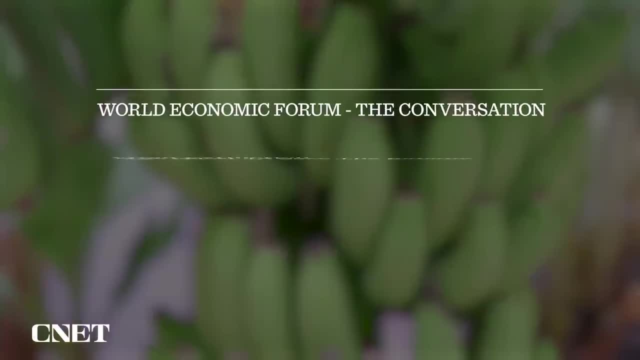 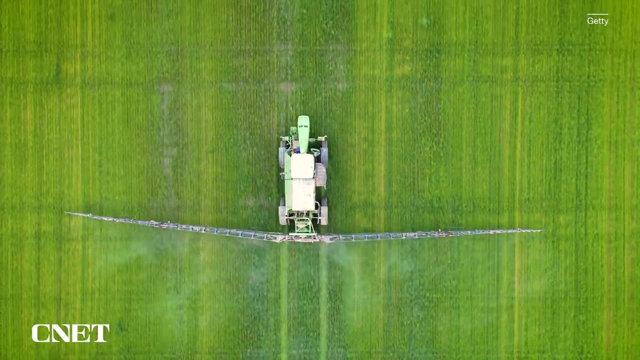 destroying the food supply of potatoes, And that's why the growing banana plants from Asia to Africa, because of our heavy reliance on a single banana variety, Diseases, pests and a volatile climate can all threaten the viability of our food supply, As farmers grow and harvest fewer varieties of plants and 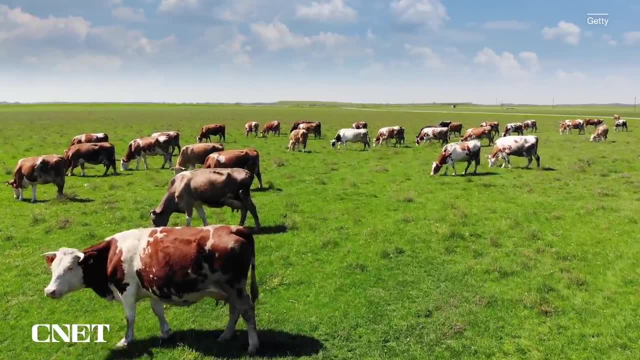 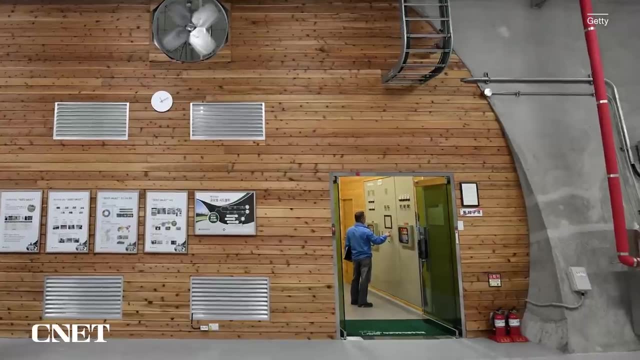 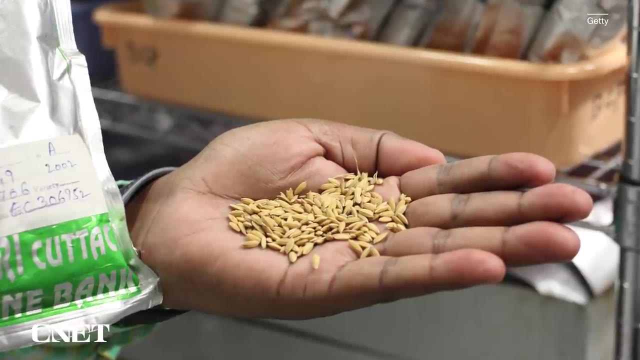 animals, the global food system could become less resilient. Greater agricultural resilience means restoring endangered crops and food varieties. Seed storage facilities play an important role in preserving the seeds of wild and natural and domesticated crops. Seed vaults act as an insurance policy for the world's food supply, offering backup plans for future. 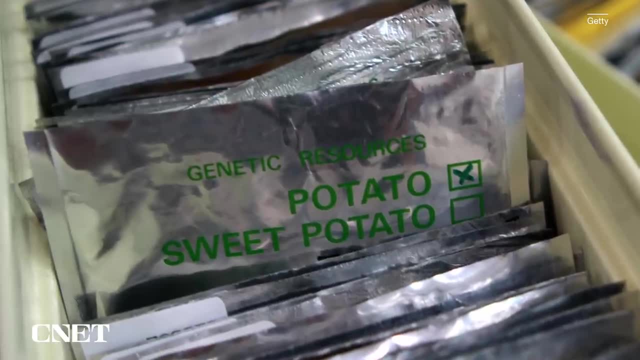 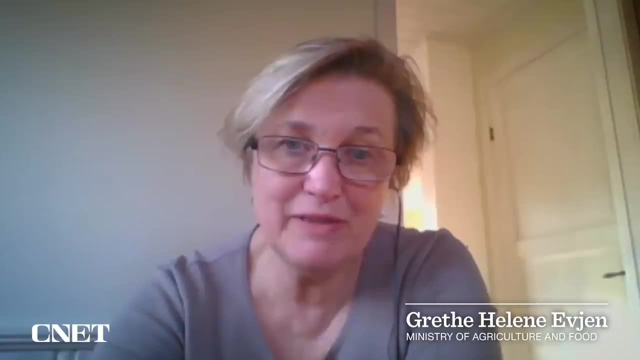 generations to overcome the challenges of climate change and population growth. My name is Greta Helene Evgen. I'm working as a project manager for the Svalbard Global Seed Vault. The Svalbard Global Seed Vault in Norway is the largest seed. 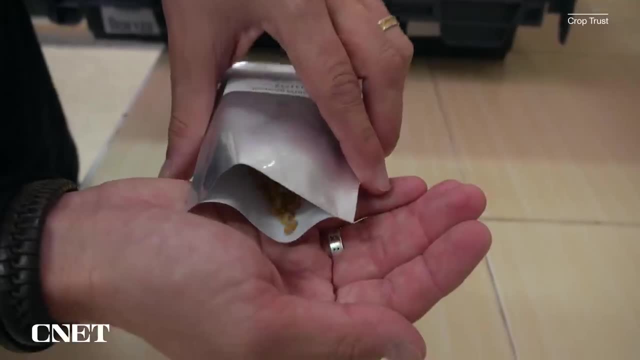 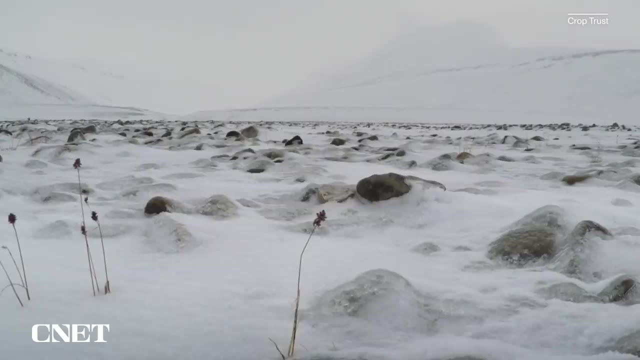 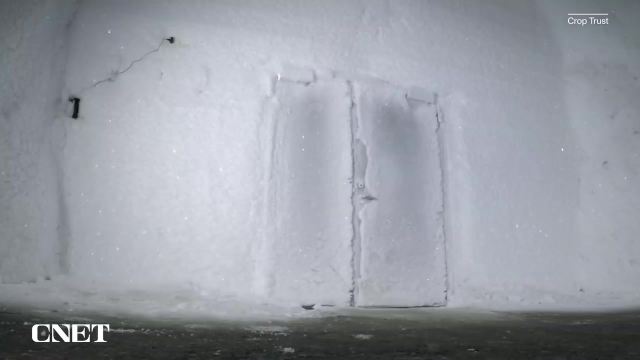 storage facility in the world and houses more than 1 million samples. Like most seed storage facilities, seed storage facilities are based on permafrost, a layer of frozen soil, to ensure that seed samples remain intact even if the facility loses power. Permafrost, like the name suggests, acts like a giant freezer. 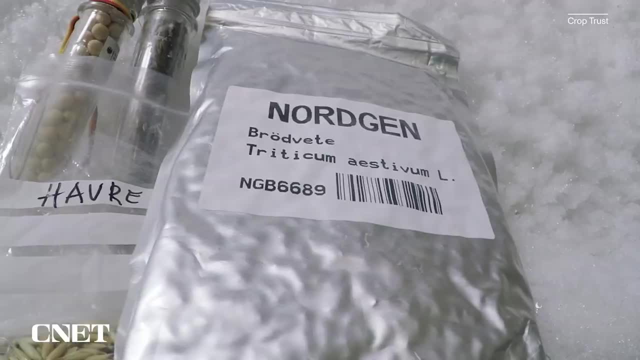 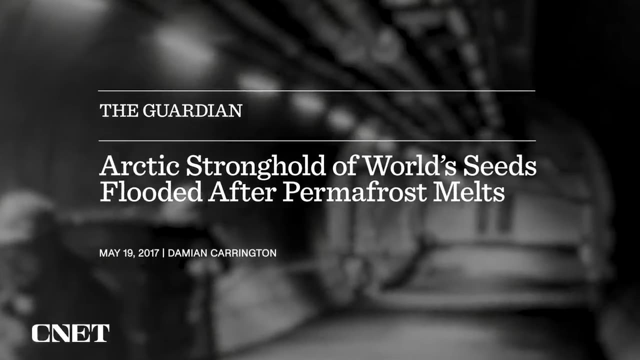 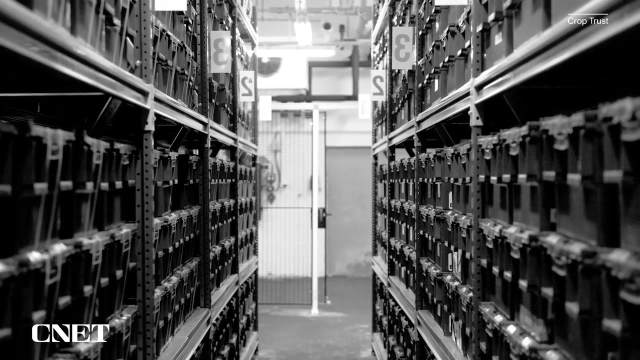 keeping microbes, carbon, poisonous mercury and soil locked in place, But it's not always a foolproof system. In 2017, rainwater gushed into an entrance tunnel and the facility flooded. Fortunately, no seeds were lost, but the event demonstrated that the permanence of frozen ground is no. 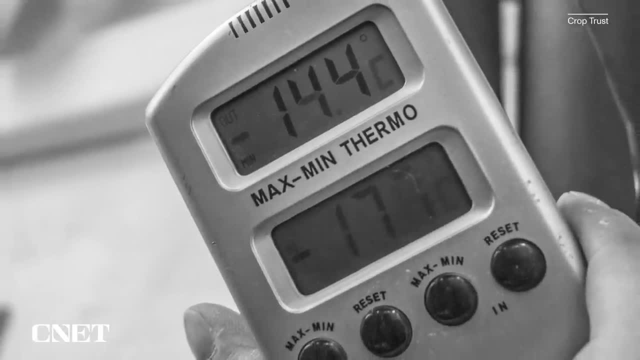 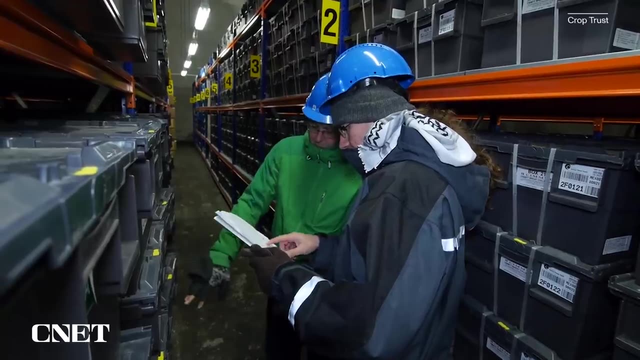 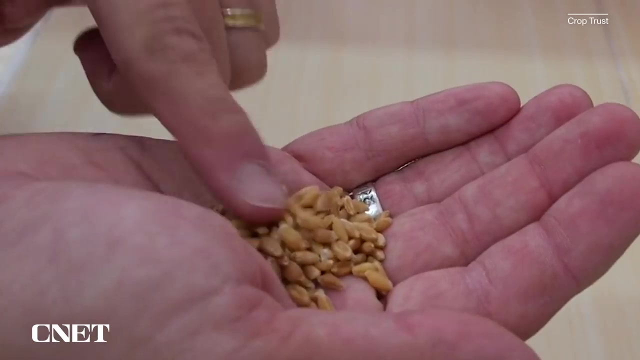 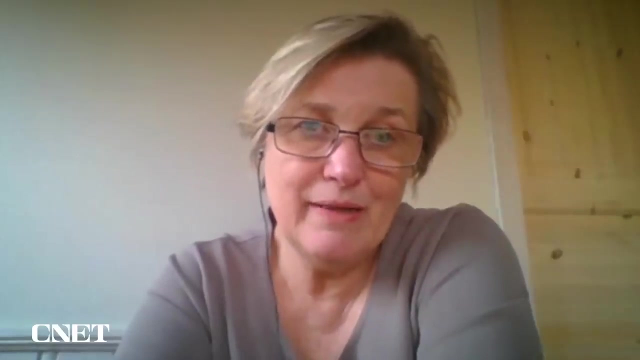 longer guaranteed. as Earth's temperatures continue to climb, Gene banks are vulnerable to many different things that could happen to them If they are left with no electricity and they are placed in warm areas. the seeds will lose their viability after a really short time And they have been flooding and could be fire that destroy the 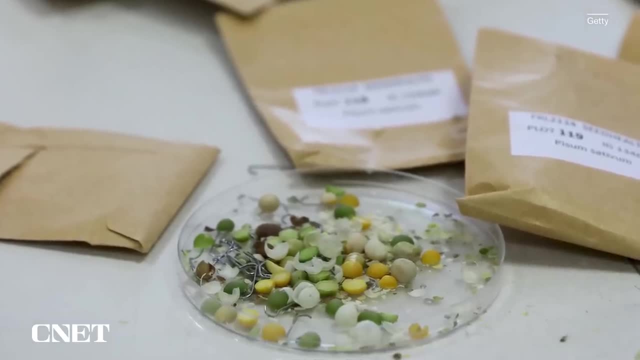 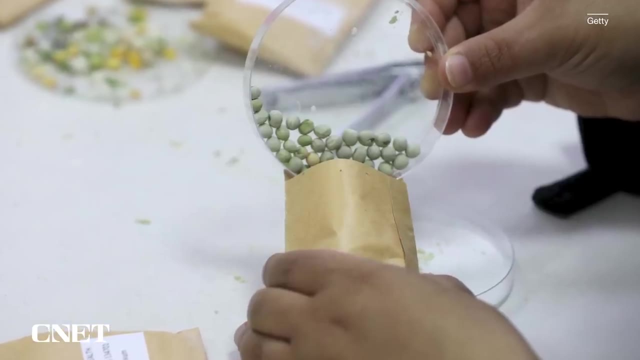 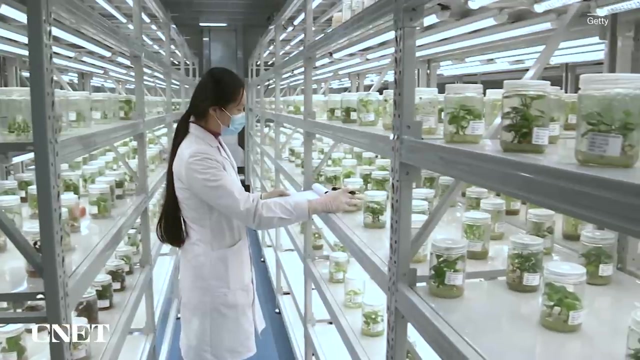 facility. So it's really important for those gene banks to also have some copies placed in other areas. Seed vaults not only store and protect a diverse collection of plant species, they're also gene banks, an important resource for researchers, horticulturalists and conservationists looking to experiment with the 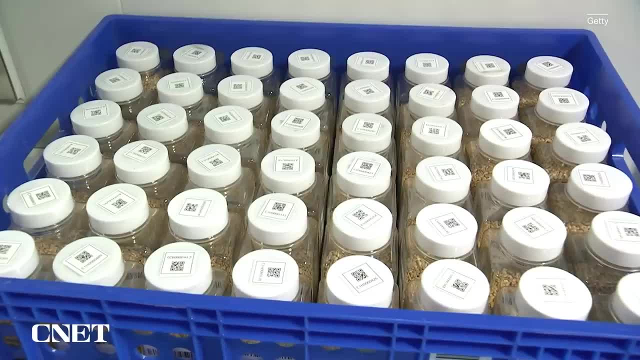 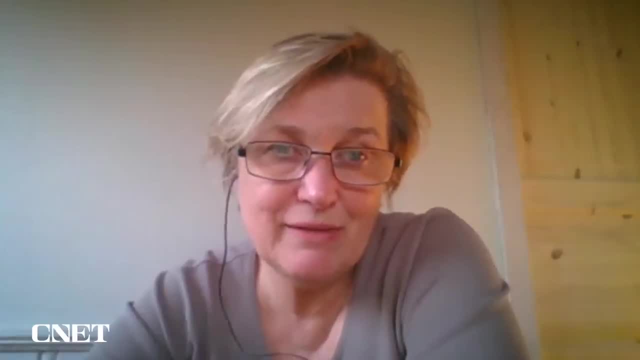 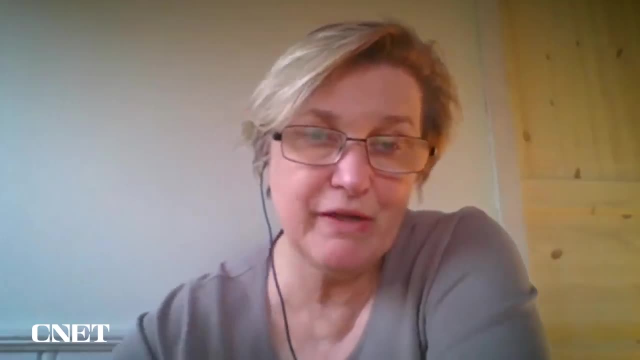 genetics of a particular plant species, The gene banks that are located all over the world. in each country they provide the seeds. So researchers, the breeders and even to the farmers that would like to experiment or to see if they can find a new variety that have some specific 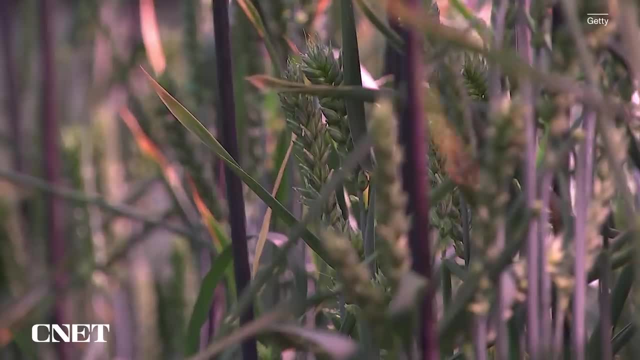 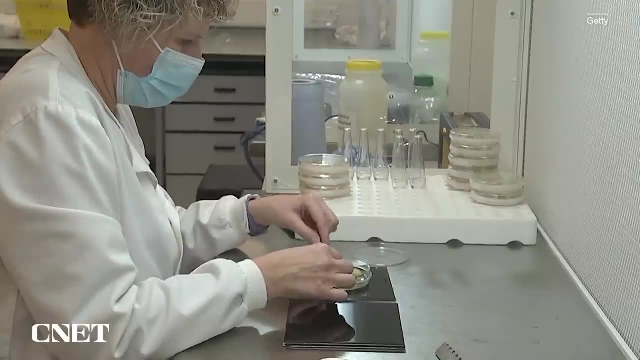 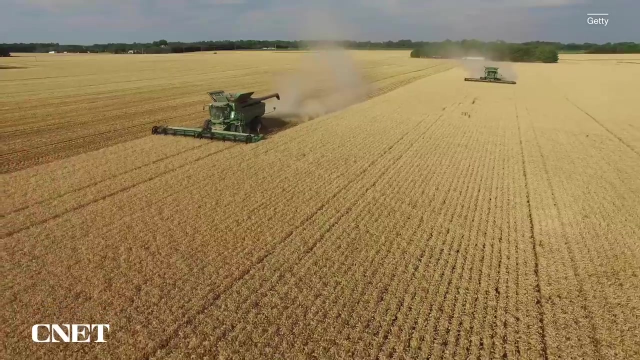 growing features And I think that's a growing interest in many countries that more and more people would like to experiment and to learn about diversity and what you can get from diving into the genetic diversity inside the seeds. Today's real model crops wither in the face of climate change, drought and 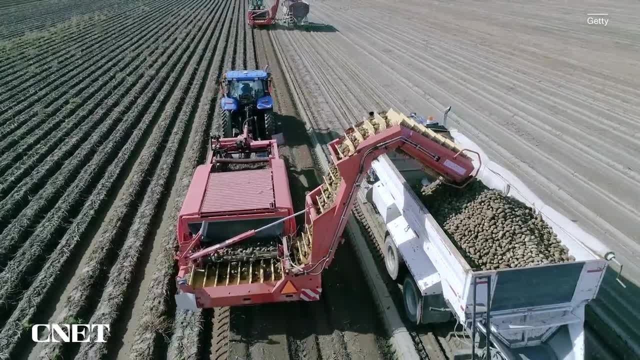 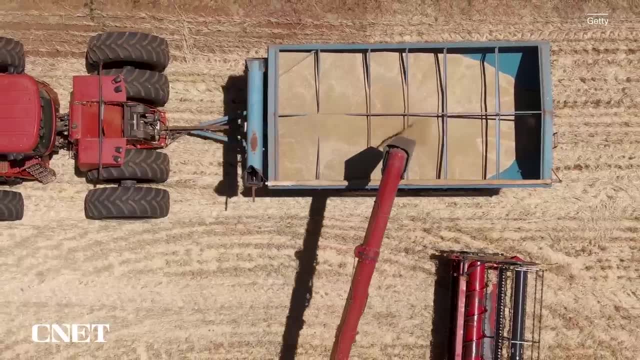 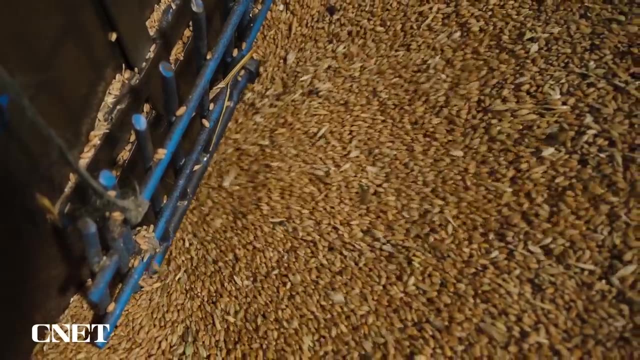 emerging diseases, forcing farmers and plant breeders to look for crops with traits suited for a changing planet. Experts say saving endangered crops is vital in a future already facing challenges: to feed a growing population, reduce emissions and find fresh water. In addition to gene banks, advances in technology also offer solutions to 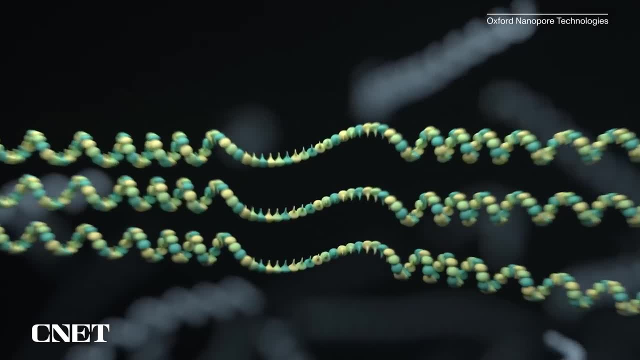 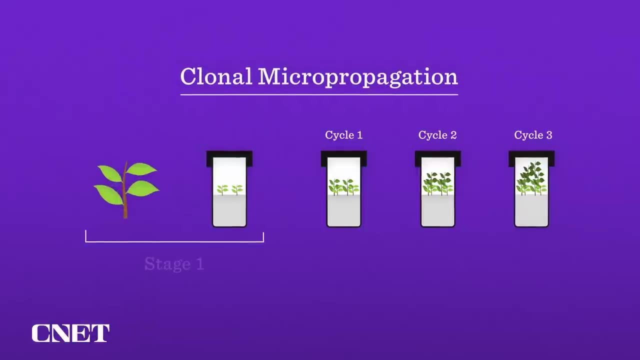 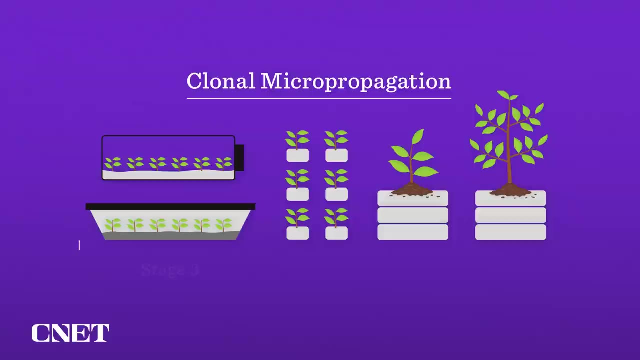 saving crops facing extinction. Scientists can breed crops To sustain extreme weather conditions and to better adapt to their changing habitat. Clonal micropropagation is a technique that involves placing plant tissue in a flask with sugar and nutrients under artificial lighting inside the vessels. 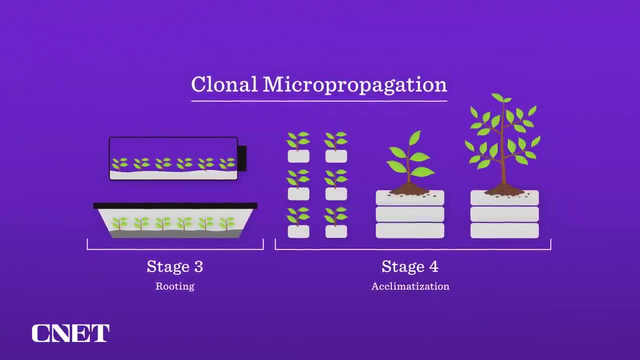 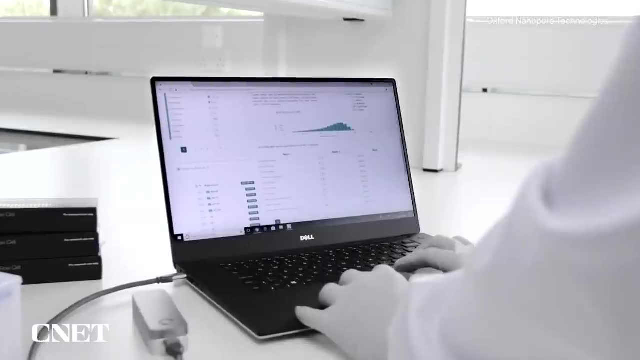 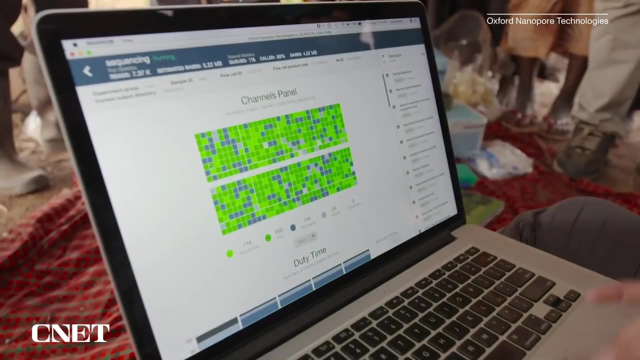 The plants are grown on culture media that contain nutrients and growth regulators. The minion DNA sequencer provides real time DNA analysis in remote areas. The technology is still in early days, but these devices could help scientists quickly identify plants in the field and cross-reference them against taxonomic catalogs. 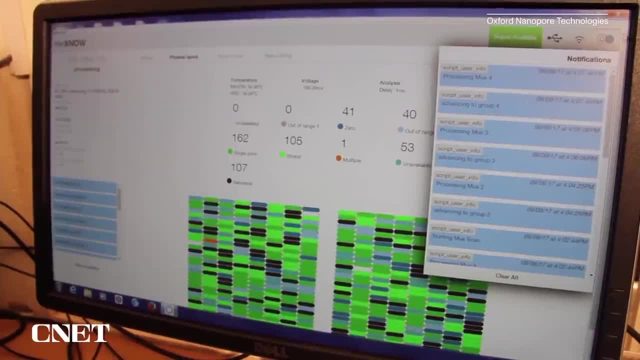 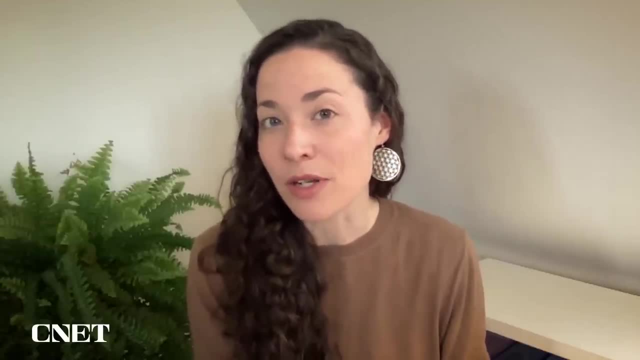 That way, they can better identify if a plant they've stumbled upon is threatened by extinction. A genetically homogenous crop, which is a state that characterizes a lot of the things that we grow in in industrial production, is one that is also genetically vulnerable. 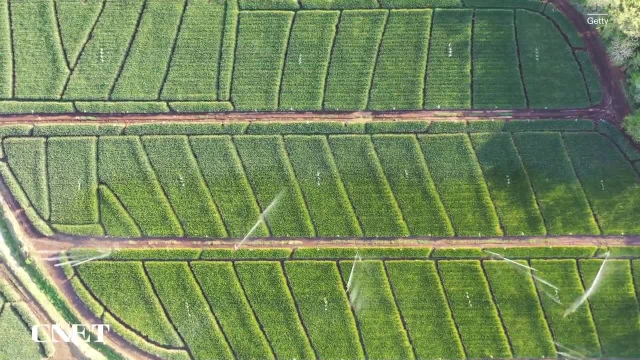 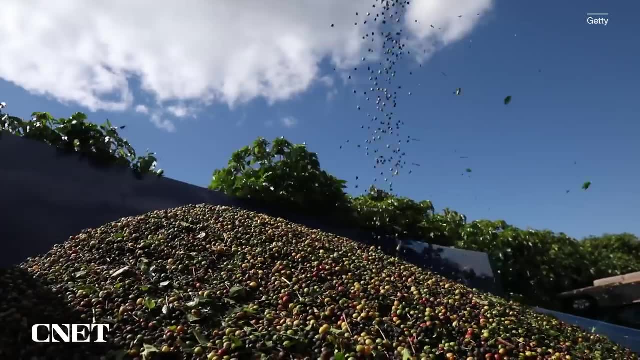 And in that sense we might also in some cases, think of our industrial crops as being endangered. in a way, They're endangered If we don't have the resources available in order to push them in new directions in the future, or if there are new. 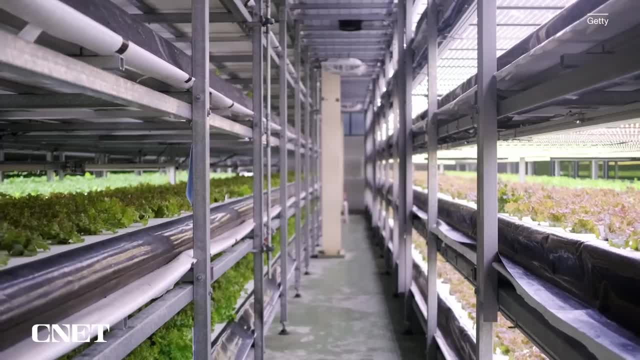 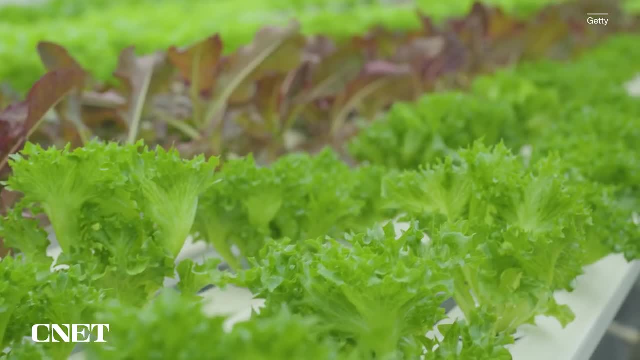 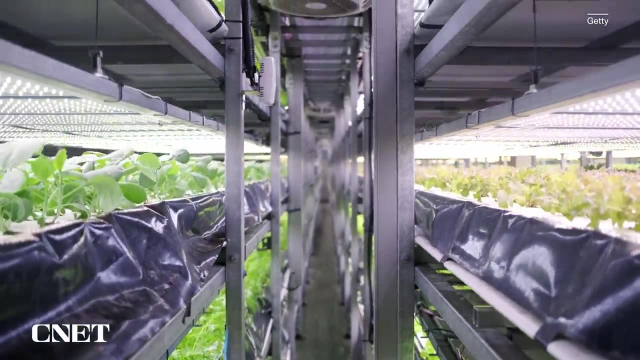 demands put on agricultural production. Vertical farming is the agricultural process in which crops are grown on top of each other rather than in traditional horizontal rows. Growing vertically conserves space, often producing higher crop yields per square foot of land used. Diversifying the crops we eat and adapting crops and crop production to be more.